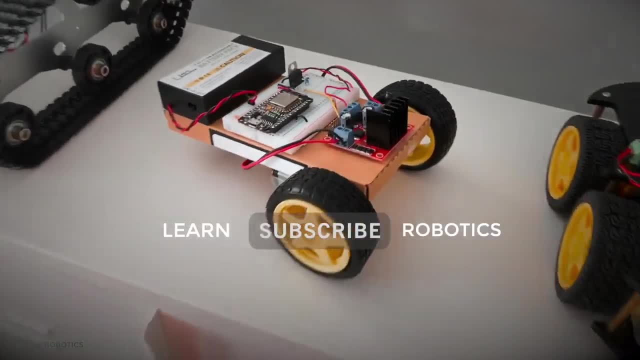 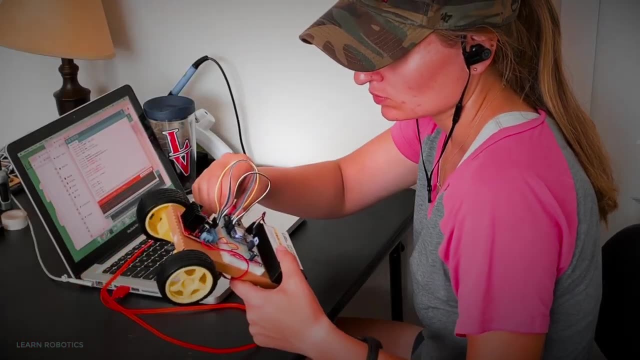 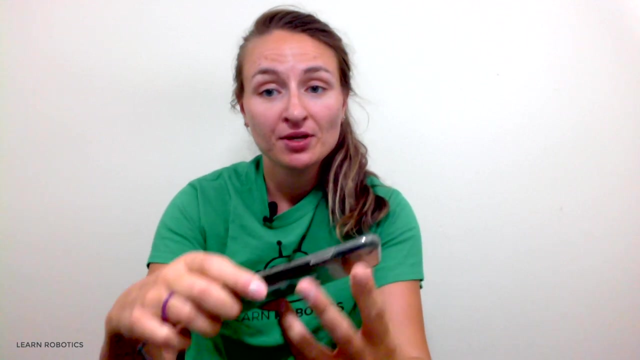 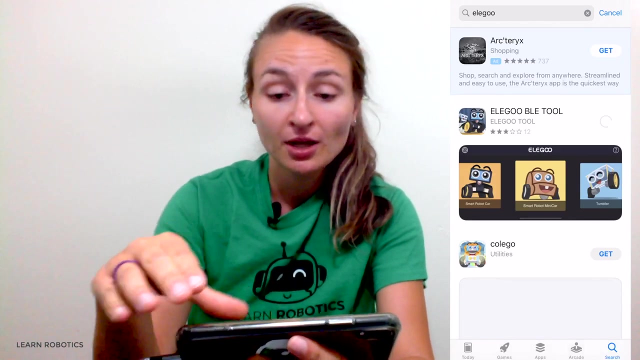 face. So the first thing you're going to need to do is download the Elegoo app. It is available for iOS and Android 100% free. All you need to do is search Elegoo and it should come up So once. 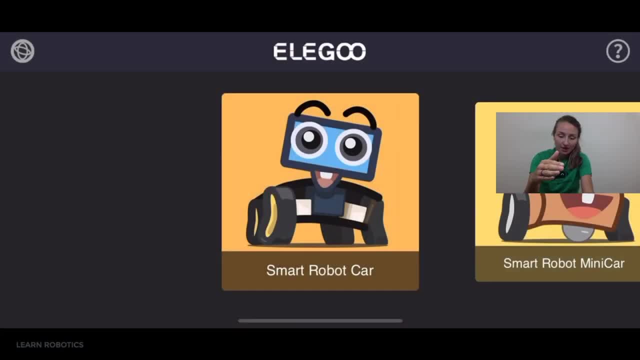 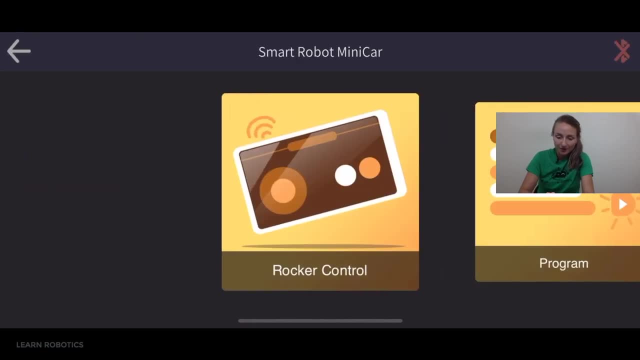 you have the app. we're actually going to go take a look at it right now. You can launch it, And we've got the smart robot minicar, So you're going to click on that, And if you have some of the other cars that they offer, I'm a huge fan of their Elegoo. 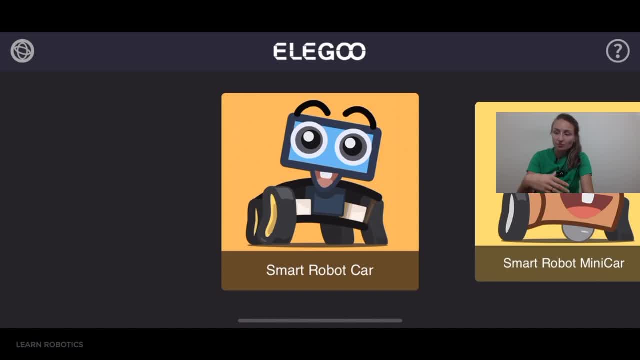 Smart robot car. I use that in the Build Arduino Robots course. I also have a few tutorials using that. They've also included that here. So if you're an Elegoo fan or you have some of their other products, they have updated this app and you can also control that robot using this app as. 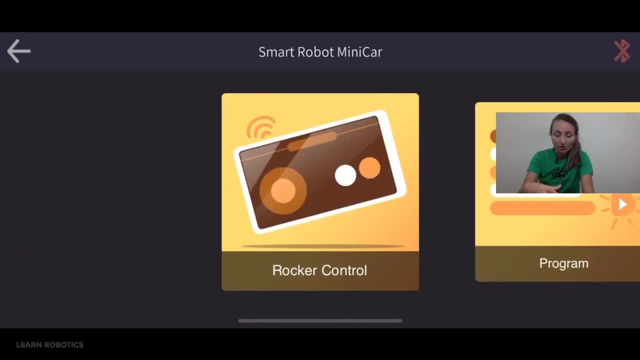 well, But for now, we're just going to head on over to the smart minicar And what you're going to need to do is have your robot charged and nearby. I'm going to show you what this rocker control is going to do. And I'm going to show you what this rocker control is going to do. 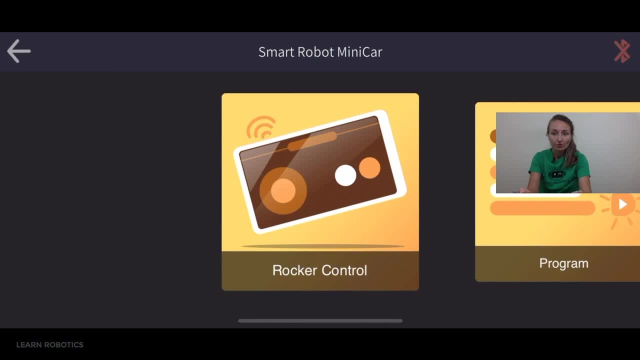 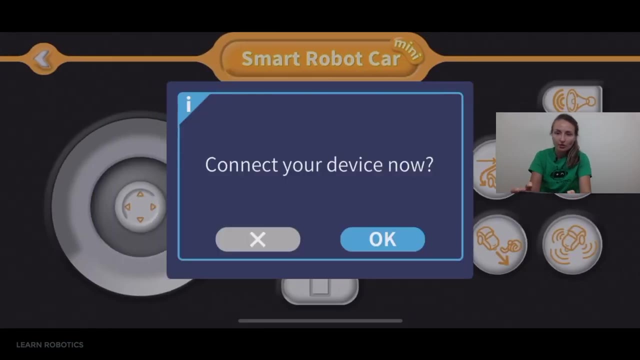 It's basically like turning your smartphone into an RC controller for this robot, So it's pretty cool. So we're going to flip on the on switch on the car And it should light up, And then we'll click on rocker control And it's going to ask you to connect your device. Just make sure your 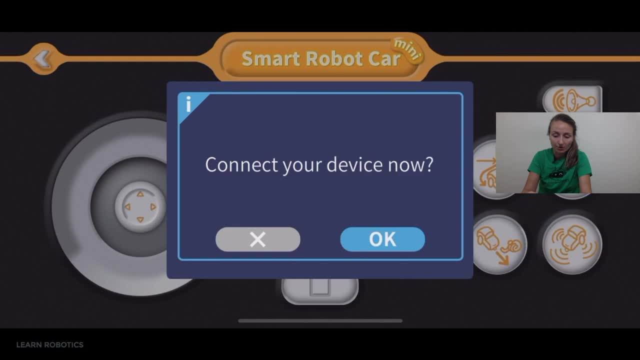 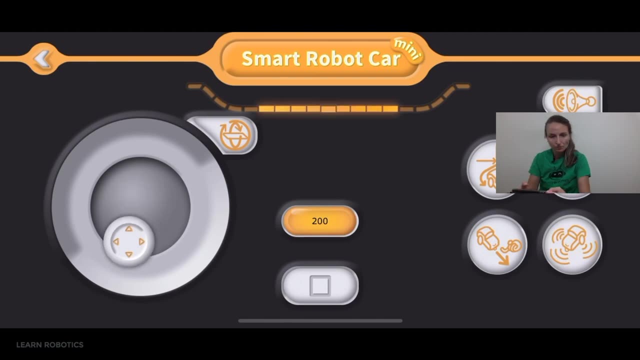 smartphone has Bluetooth enabled. Otherwise it won't be able to connect to the car. Just click OK And we're connected. So now we can actually drive our robot around. use the joystick to control the motors, And you can also use the gyro on your phone to control the robot as well. So we'll go ahead and we'll shut. 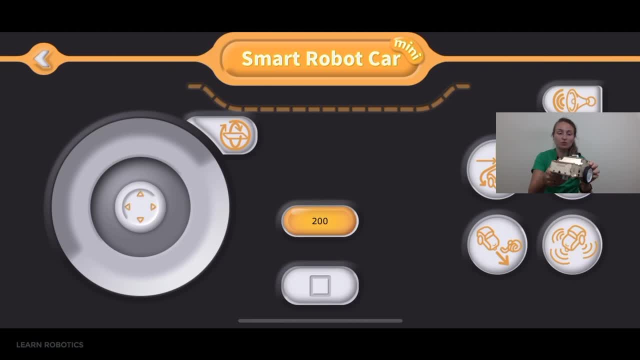 that mode off. Another cool thing to know is that this little Jeep has a speaker or a buzzer, and you can actually trigger the horn. So that's pretty cool And so, literally right out of the box, you can start driving this thing. 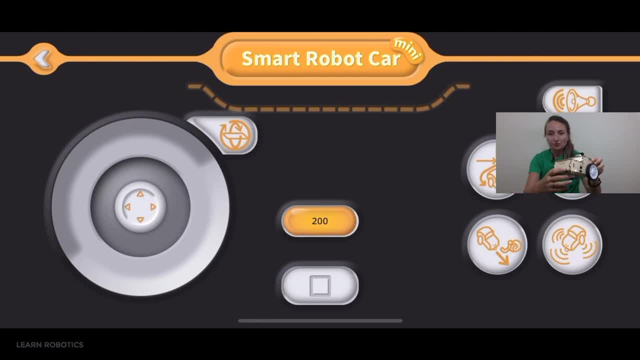 around. It's got some built in modes. you can do some object avoiding, object following, you can do line following. So it's pretty cool, Already pre programmed, And what we're going to do is we're going to actually explore some of those topics in this lesson and learn how they're actually 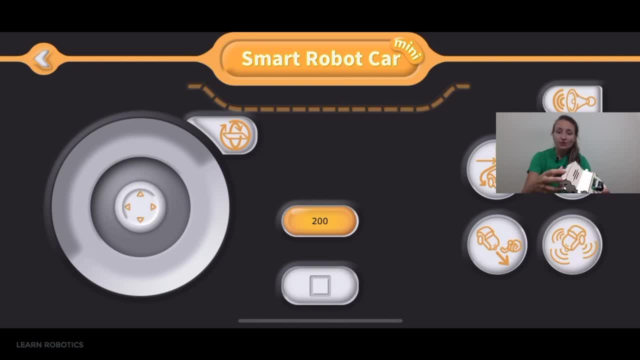 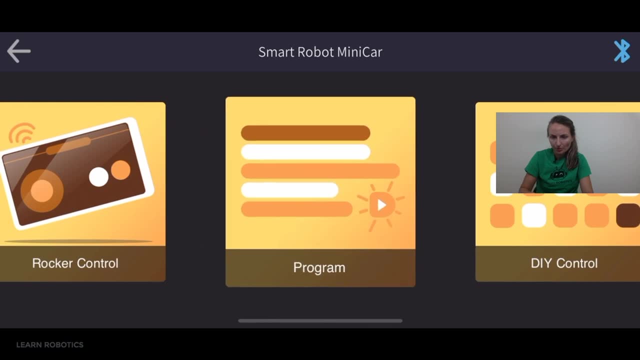 designed these programs, put together our own simple program And then we're going to go ahead and we're going to do a simple program using obstacle avoidance. So let's head on over to the programming menu And you'll see. if you're familiar with. scratches is a very similar setup. 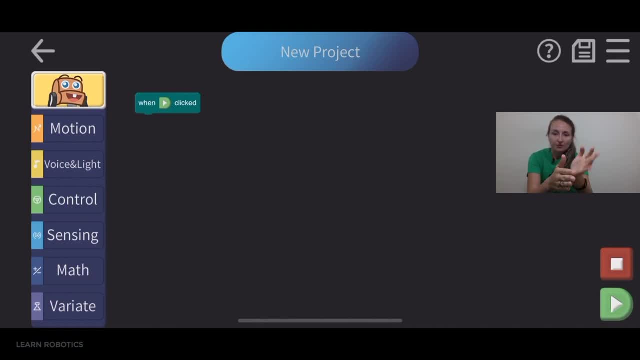 you've got a bunch of different categories on the left, And then on the right you've got your actual programming board where you can drag and drop the blocks over and then you connect them. So the way the program is read is this: top to bottom, And then if it's inside of a loop it'll go top to bottom. 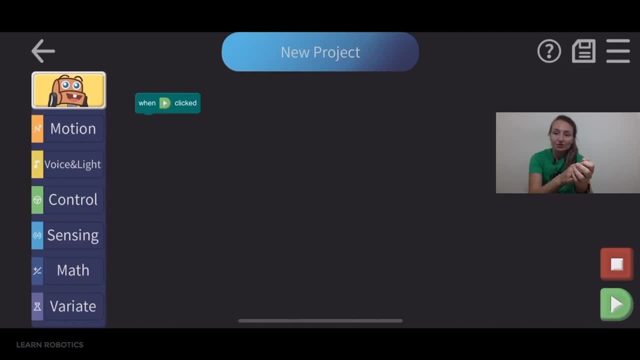 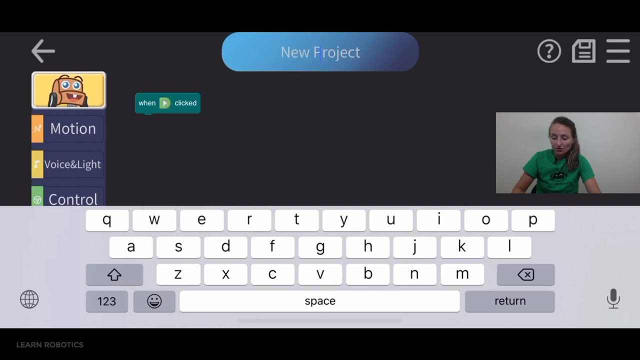 and then it will repeat itself However many iterations you tell it to, And the top is where you can name your project And I'm just going to call this. let's just call this move. We'll just do a very simple move just to kind of get. 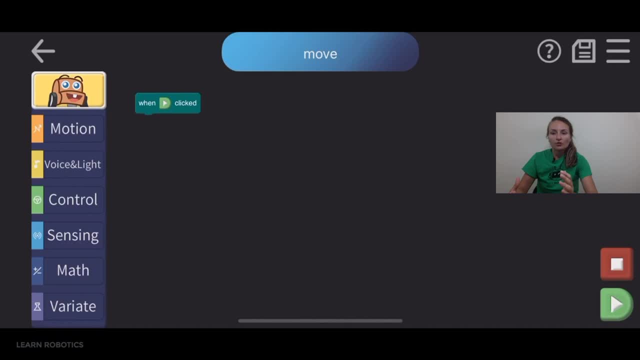 used to how the blocks work and control. So if you're more advanced with programming, this may seem like really simple, maybe unnecessary, but I always recommend, with any robot that you're working on- whether it's fair, completely simple or very complicated- to get used to it first by doing something simple, you know. 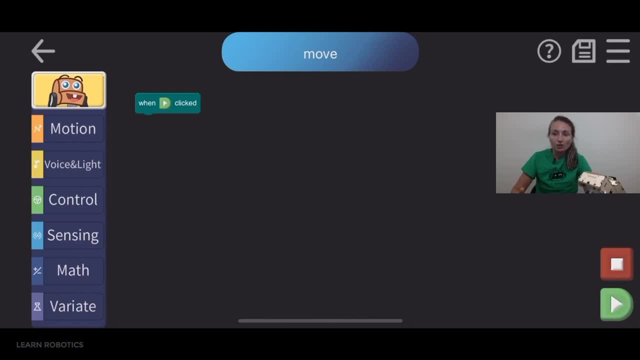 the best way to get used to how a robot moves, or even robot control, is to always have like a baseline, And so, whether I'm working on a little robot like this one or an industrial robot arm, it's always good to program something that you're familiar with and just see how it works And that 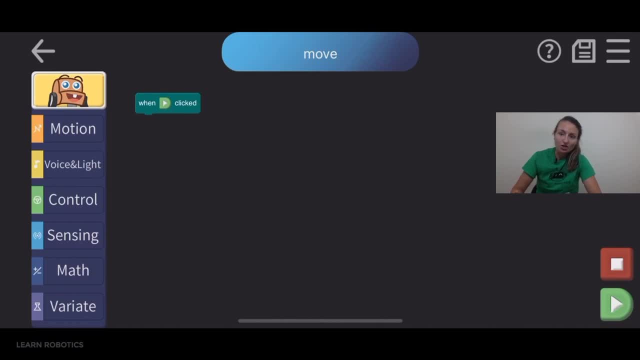 way. if it doesn't work the way you expect, You can always go back and make changes, and it's not a super complicated program that you're going to have to try to debug and troubleshoot. So let's go ahead and write a very simple program that moves the robot forward for about 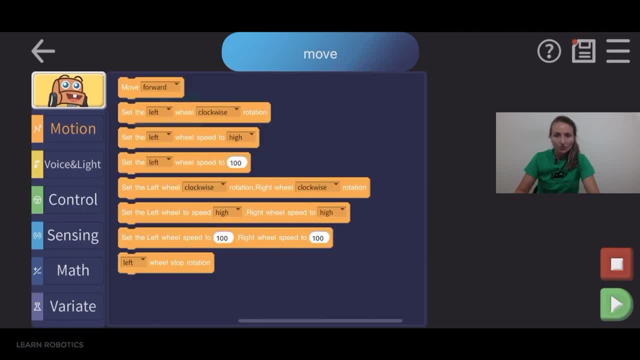 a second and then back. So, if you can see, I opened up the motion tab and there's a command called move forward and any of the commands that have like a little arrow pointing down that means that there's more than one option available. 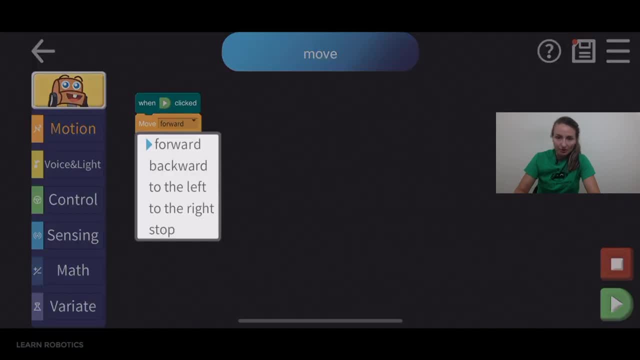 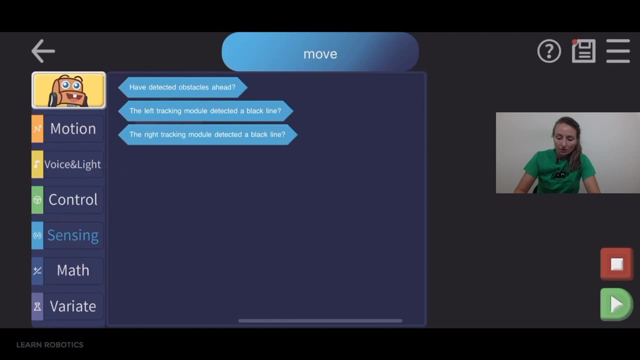 So we can go back and forward can actually be changed to backwards, left, right and stop. So what we're going to do is we're going to move the robot forward. We'll do that for one second. So open up the control window and choose the weight, and we'll just leave it at one second. 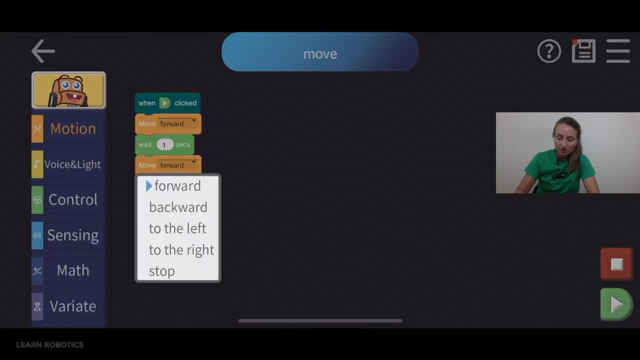 and then we're going to go back into motion, and then we'll make it backward, and then we're going to do: actually, let's just make it stop for now. So we'll drive forward for one second and then we'll stop. So what you do is you can go up to the right corner and click save, and it'll be saved in. 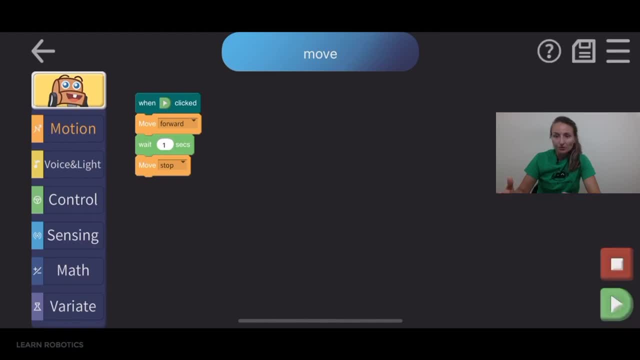 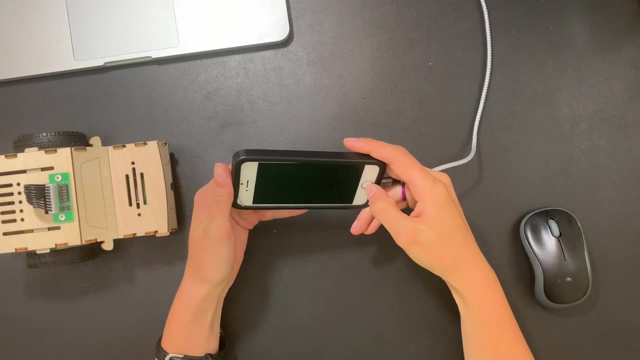 with some of your other programs, and then to run this program, all you need to do is to go into the bottom right corner and click on the green play button, So forward for one second and then stop. So what we can do Is we can go into the app and then what we'll do is we'll click the little play button and 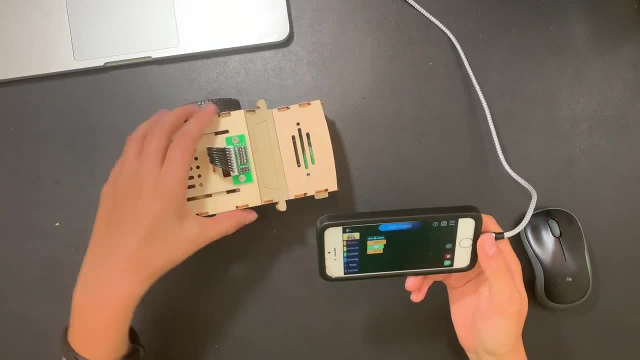 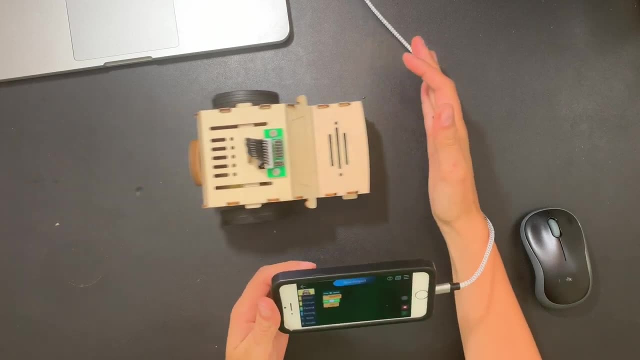 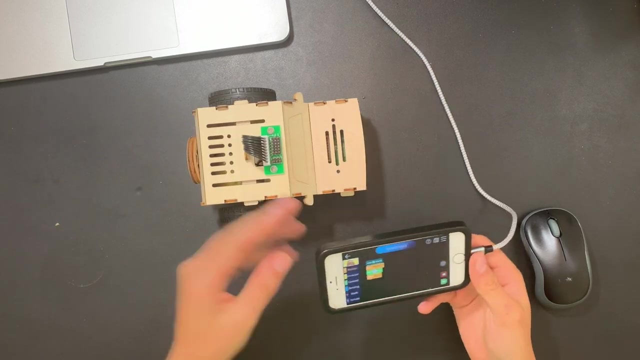 the robot should move forward and then stop. And I always recommend, if you're going to be running some more complex programs, to do the testing on the ground. That way you don't inadvertently send this guy off the table. But for this we're just going to do very simple movements. 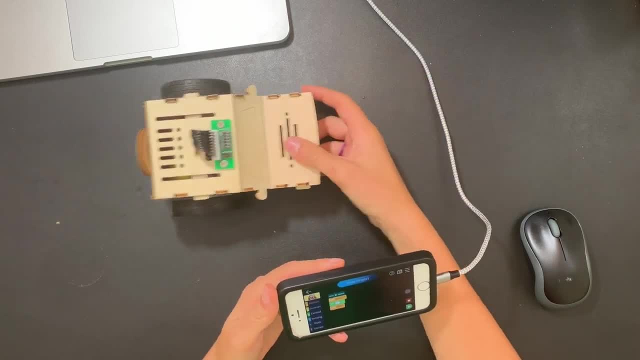 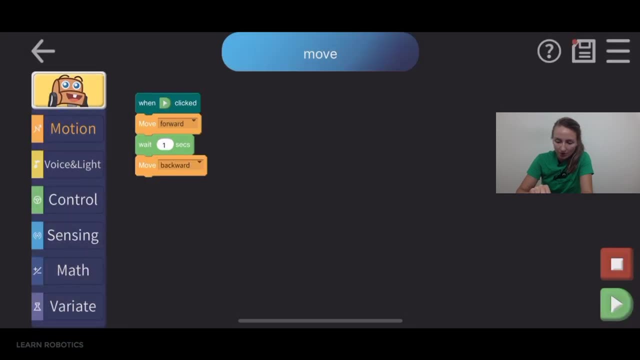 So now let's go back into the app And we can add some more Things to our program. Let's go ahead and we can make that move backwards. We'll add in another second and then we'll go ahead and we'll stop. 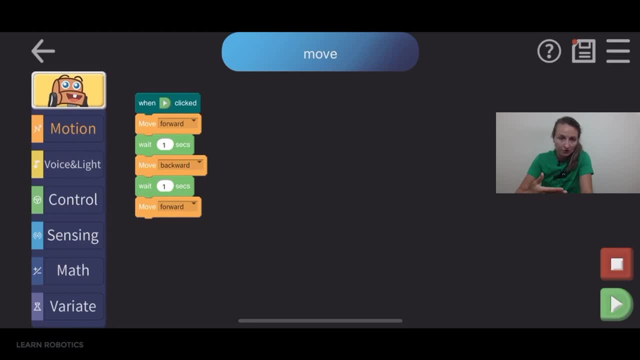 And once you get the hang of this, it's like actually pretty fun, Like you can do this, like with your friends or you, if you have kids, you can do this with them. It's kind of entertaining to go through and you've got all these different functionalities. 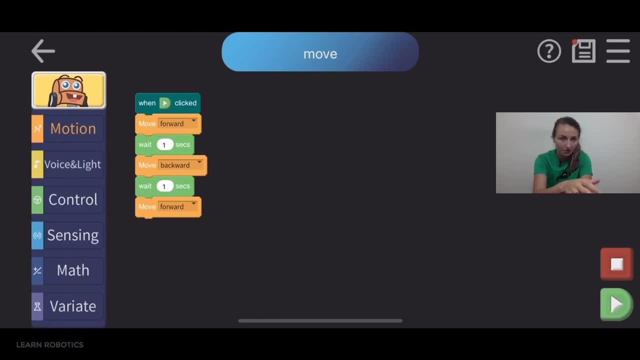 just completely built into the app. You don't need a computer. You don't really need to install any special anything Other than that. Better than the app that I came with, and the drivers and the software that it needs to connect should already be pre-installed. 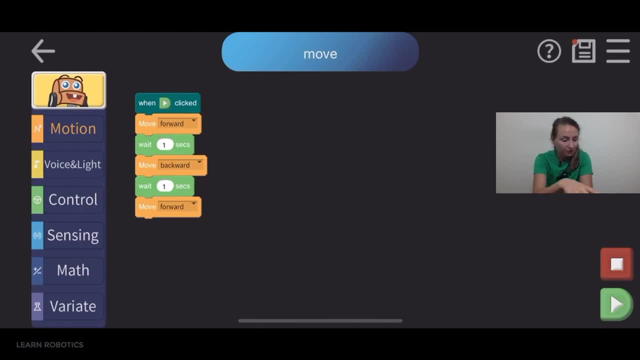 So it should be a pretty fun and accessible way to just get started with robotics. So let's go ahead and make this stop. And now we should see is when we run this program we can go ahead and awesome. So that looks pretty good. 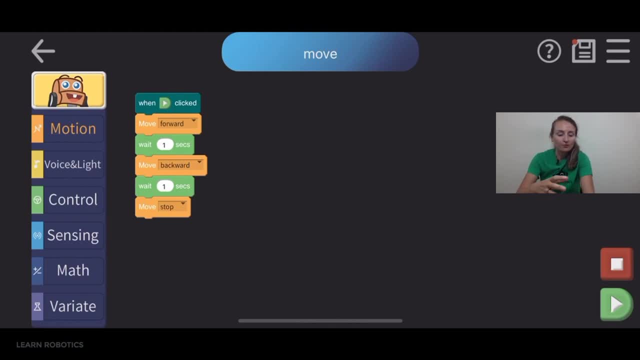 We've got the robot running. We've got the robot running. We can see what we've got. So we've got the robot running. We can see what we've got. So what we're going to do- next little project We're going to work on- is getting our robot to avoid objects in front. 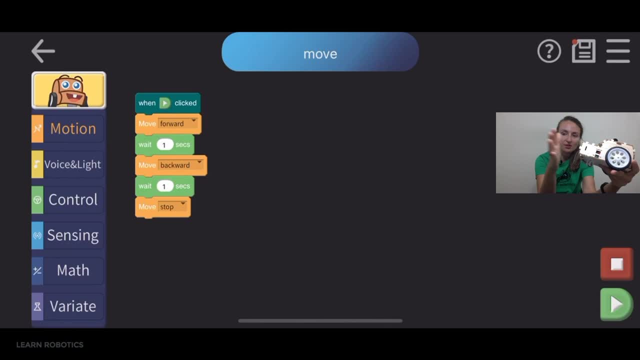 So we've got this single sensor in the front- You can see it right here- And basically, if it detects an object in the front of the robot, you can use that information to respond accordingly. And so we're going to do is we're going to detect the object. 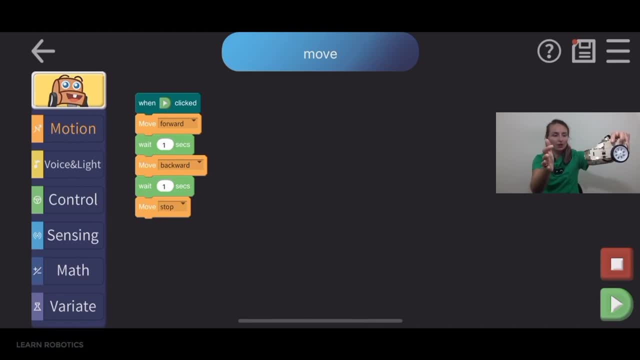 We'll stop the robot, We'll kind of back it up and then we'll like turn it around so that obviously it doesn't go in that same direction. So the generic goal: we can save the program first, create another program And then what? 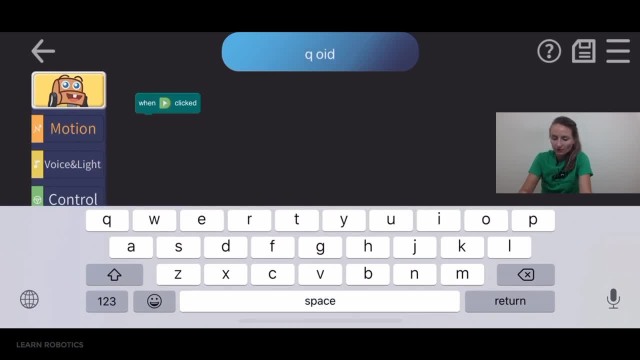 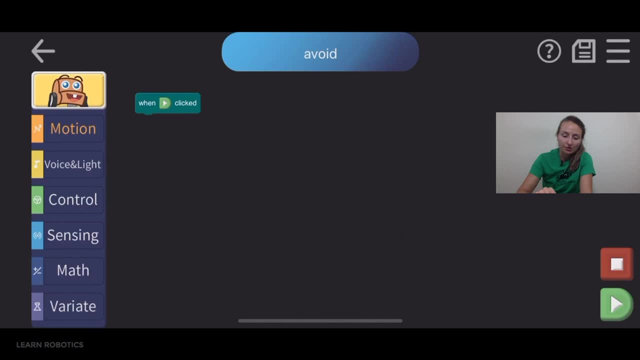 I'm going to do is call this avoid, Avoid. So the first thing we want to do is bring in our conditional, So the conditionals will be listed under control, And these are like our if statements or while statements, any sort of loops. they'll all be inside of the 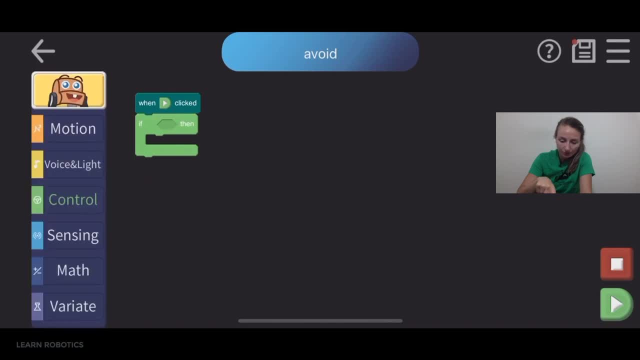 control category. So you can bring that over And then we'll use the sensing. have detected obstacles ahead. So if there is an obstacle in front of it, we can detect that and just make sure that this diamond shaped block is connected into the if statement, if it's just. 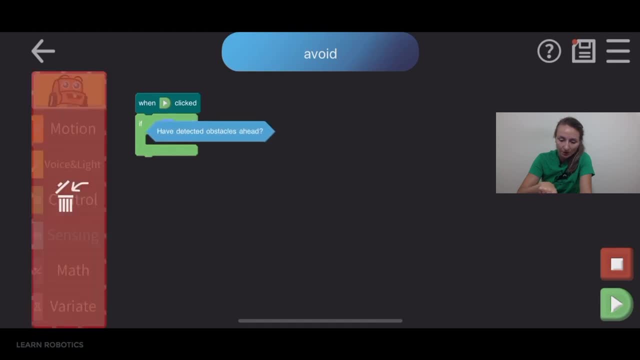 floating somewhere, then it's not going to be read. So make sure that snapped in. And so if we see the object, we're going to want to first stop the robot from moving. So go ahead and bring down a stop command And what we 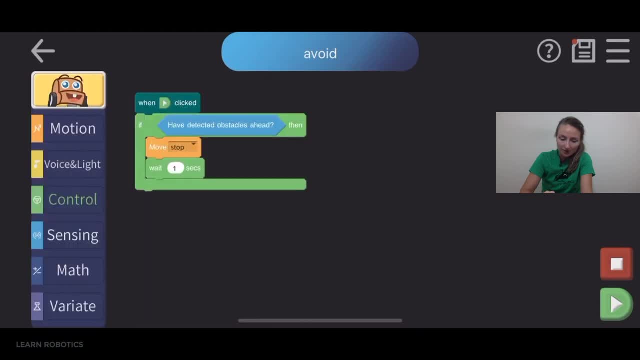 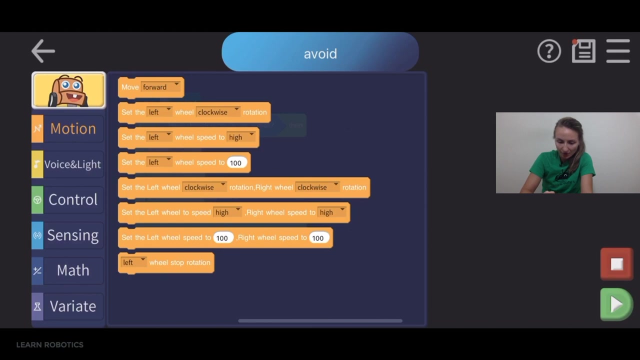 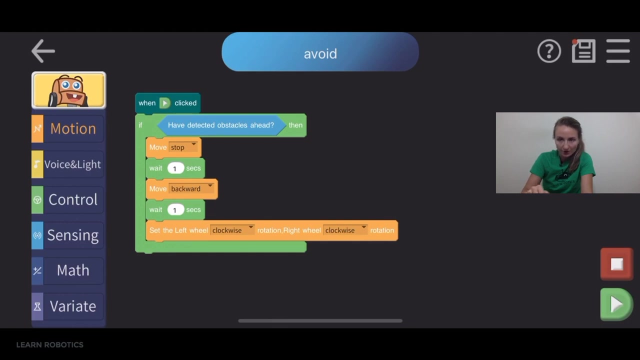 can do is wait about a second And then we can back up So we can move backwards, And then we can wait another second And we can go ahead and let's try to turn the robot. So we can set the left wheel clockwise and the right wheel counter clockwise, So whatever. 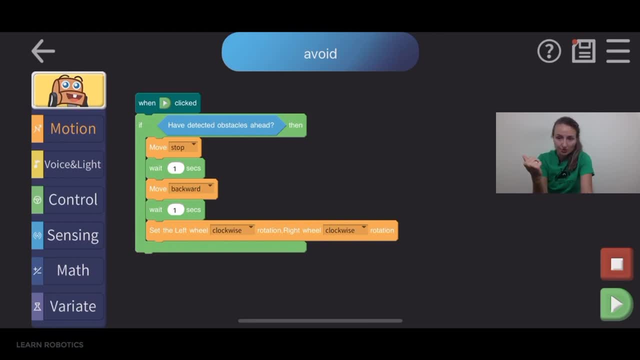 wheel is spinning backwards. that's the direction you're going to be moving in, So we'll have it. let's just have it make a left turn. So left wheel is going to be moving counter clockwise or anti clockwise, and the right wheel will be moving clockwise, So that'll be a left. 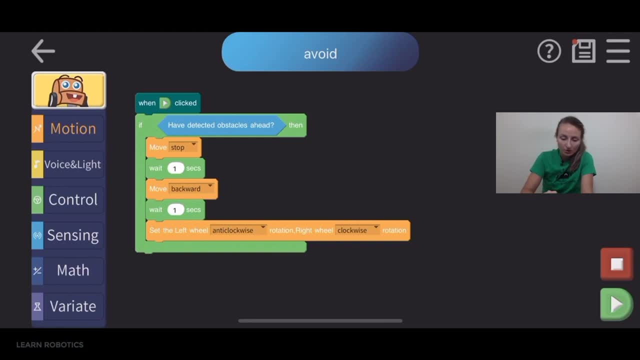 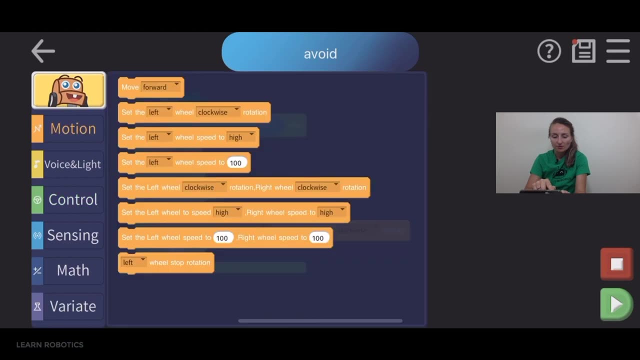 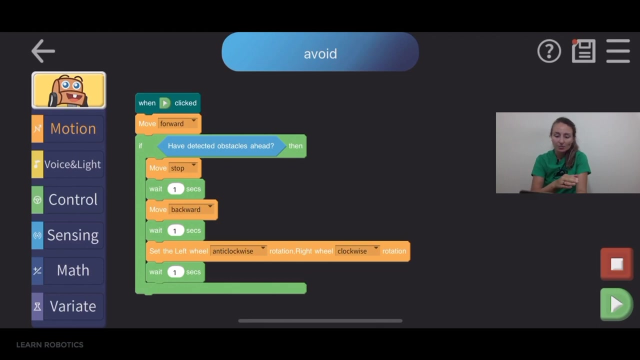 turn, And we can do that for. let's do that for about a second. So let's go ahead and just test this out. I'm going to send the robot forward before this condition happens, And then if we see an object like my hand, it should stop wait for a second move backwards. 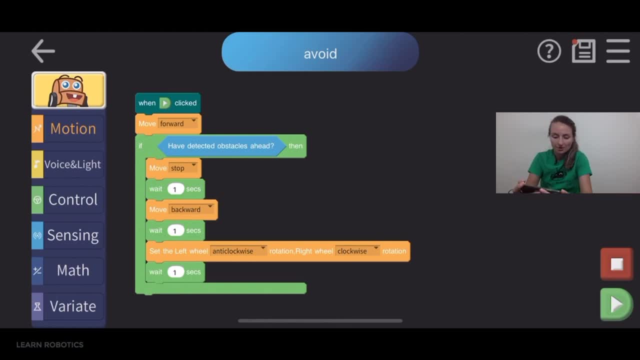 and then turn, And we should probably throw a stop in there somewhere at the end or maybe some sort of a forward motion. All right, so we can see if there's another type of a motion that we can use. It's a little. 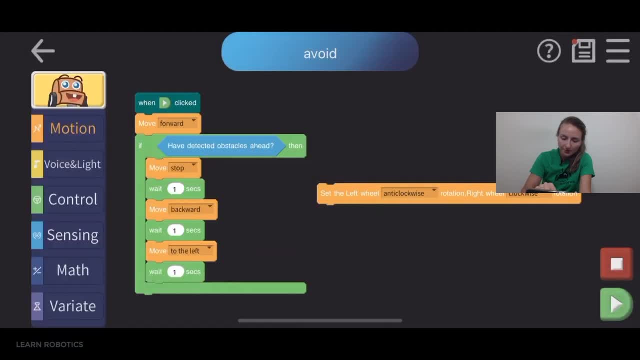 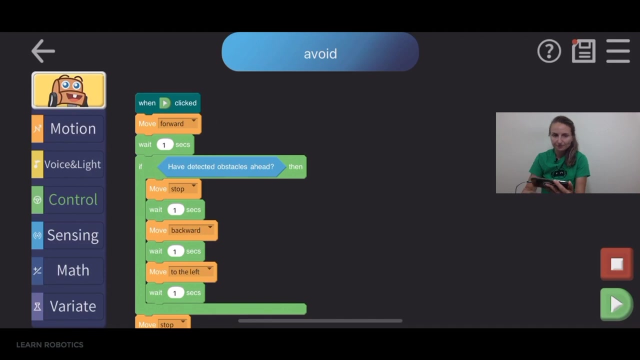 more. Here you go to the left, And let's get rid of that. We can go forward again. And then let's- let's actually just stop after we, after you, move left, Okay, so that's not bad. So let's make this go for one second And you can see kind of. 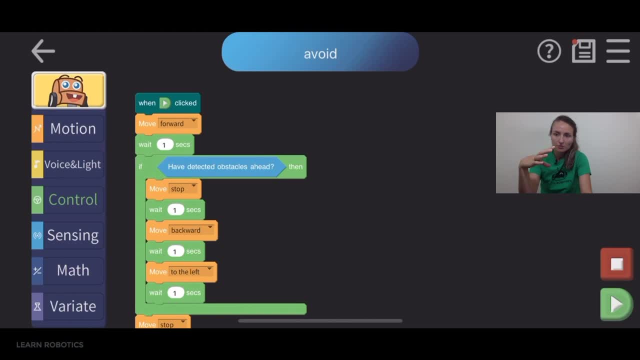 the process of going through. this is like testing out a few commands at a time and seeing if it does exactly what you want it to do And then, once it does, you can go through and add a few more things to it and make it a little bit more complex. So right now I'm 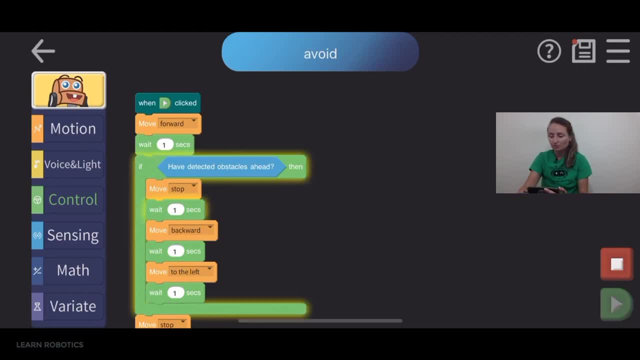 just testing to see where we're at. So now it's working Okay, so that's not bad. So let's make this go for one second And you can see kind of the process of going through. this is like testing out a few commands at a time and seeing if it does exactly what you want it to do. Okay, so that's not bad. So let's make this go for one second And you can see kind of the process of going through. this is like testing out a few commands at a time and seeing if it does exactly what you want it to do, And you can. 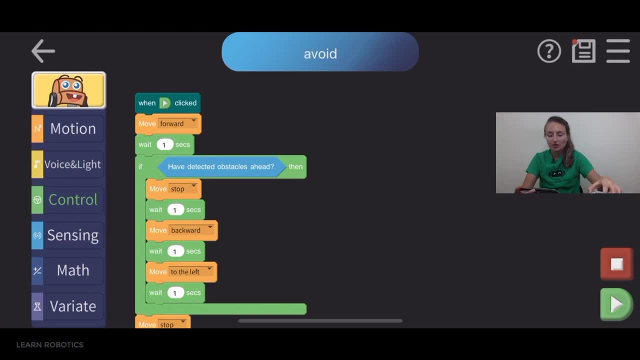 see kind of the process of going through. this is like testing out a few commands at a time and seeing if it does exactly what you want it to do. Okay, So now we're ready to get going forward again and we're not in the way of this object, So that's pretty cool. 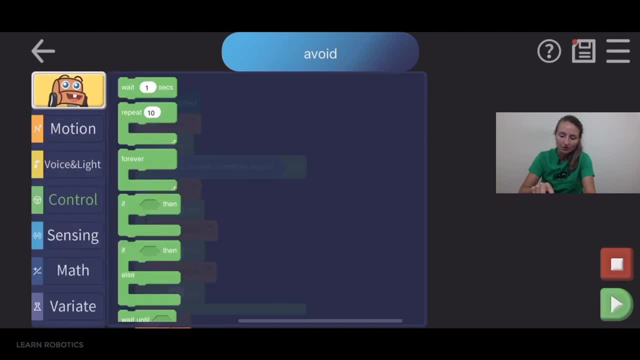 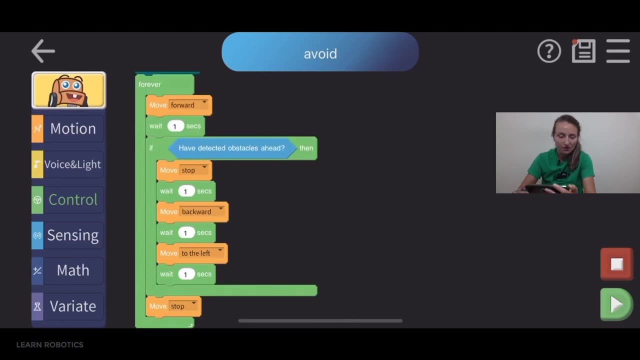 So what we can do now that we have this code is, if we want it to run forever, we can just bring this forever loop in. That's pretty nice. We've got a full set of code inside of here, So now we're basically doing object avoiding forever, And there's a ton of different. 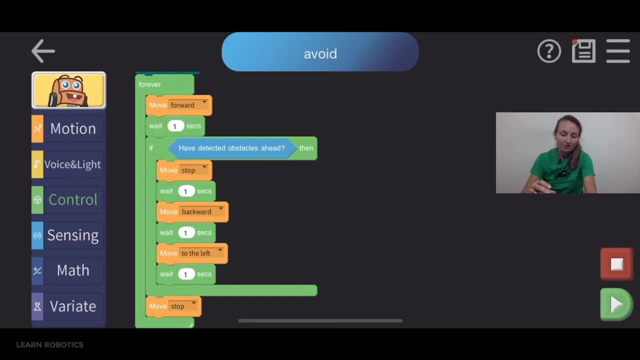 ways of doing this. You can consolidate this by not having so many nested conditions or so many steps in between, but I just wanted to show you a different way of solving the same problem. So if you were to do this object avoiding and somebody else were to do the object avoiding, 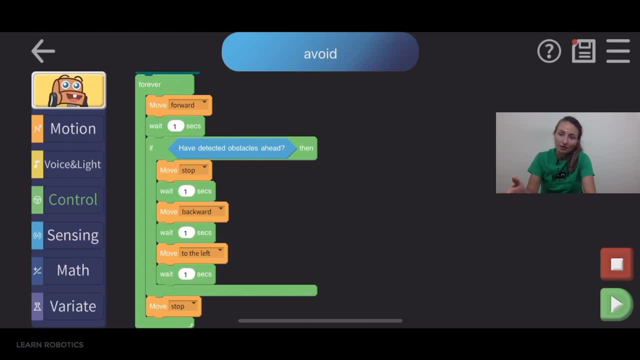 you'd probably have two very different solutions that do the same thing. So what I recommend doing is, if you have a robot available, to go through this process yourself and come up with a solution for avoiding the objects. You have access to the sensors directly with the blocks, and you have access to the motors. 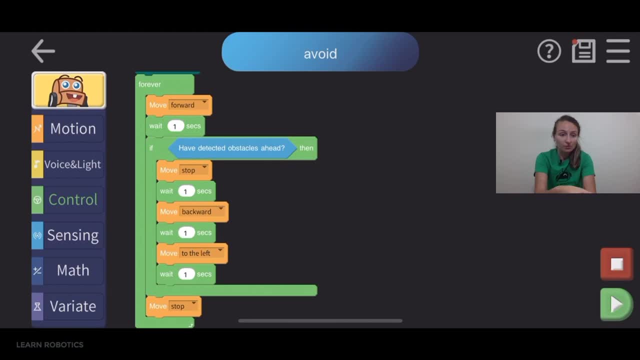 So, just basically, what you need to do is come up with the logic of solving the problem, And this is going to prepare us for next week, when we actually go through and write the controller for our DC motors and reading in the data from the sensors to avoid objects. 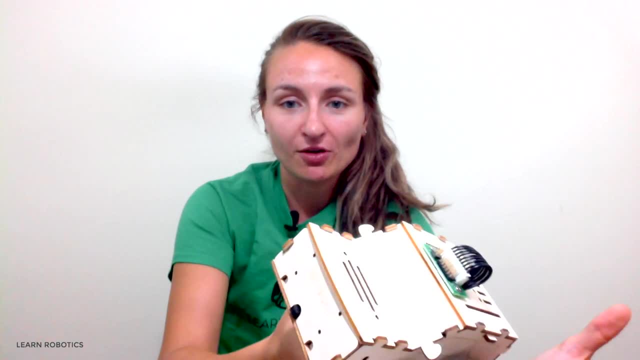 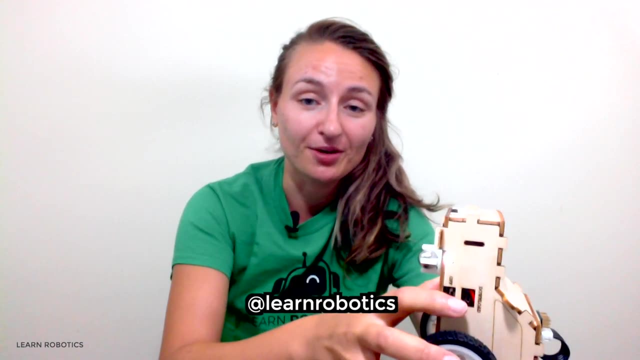 So I hope you guys had a lot of fun with this project. If you have any questions at all, feel free to leave a comment below this video or find me on social media at Learn Robotics on Facebook, Bye and Instagram, And I hope to see you guys in the free robotics course. 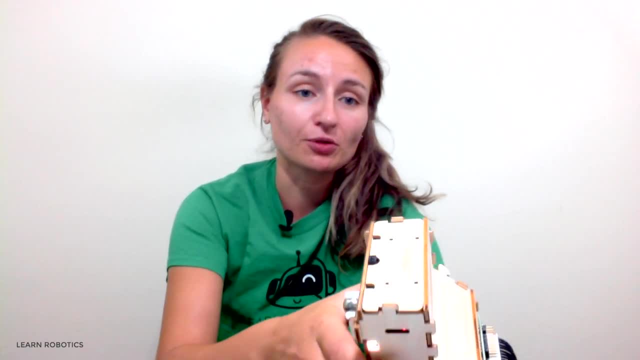 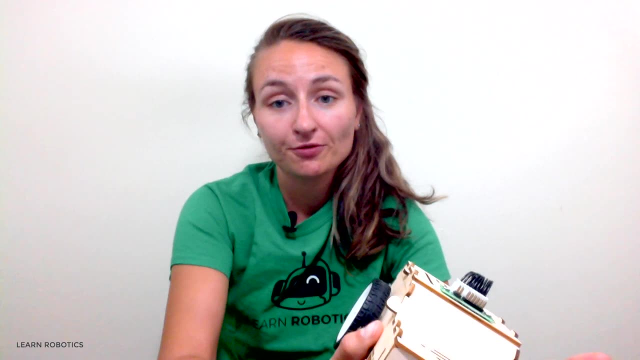 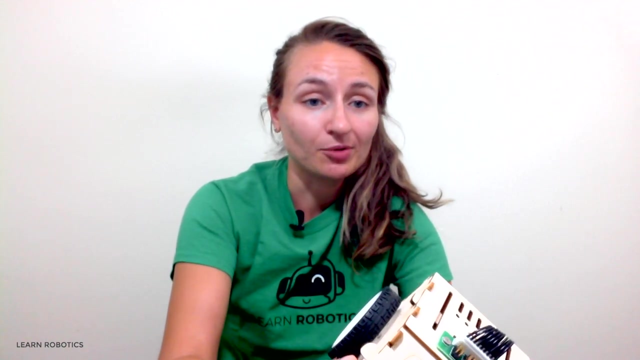 We're on episode number four. We're halfway through the first season of Learn Robotics Live, So if you did miss the previous episodes, head on over to learnroboticsorg and sign up for the free robotics class. You can rewatch all of the episodes, get access to the course, downloads, code samples and. 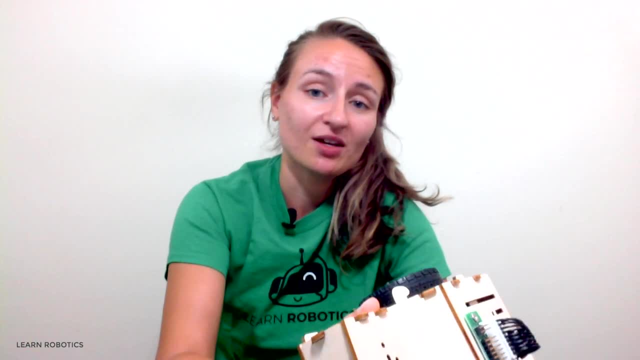 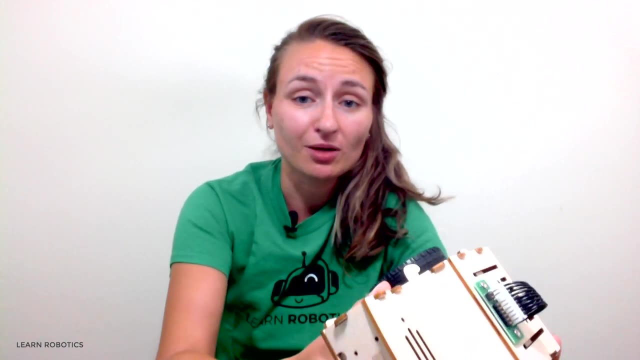 then the course certificate that I'm going to be giving out at the end of the season. So if robotics is something that you're interested in But you're not really sure how to get started, This is a great primer way to get involved with robotics at your own time.